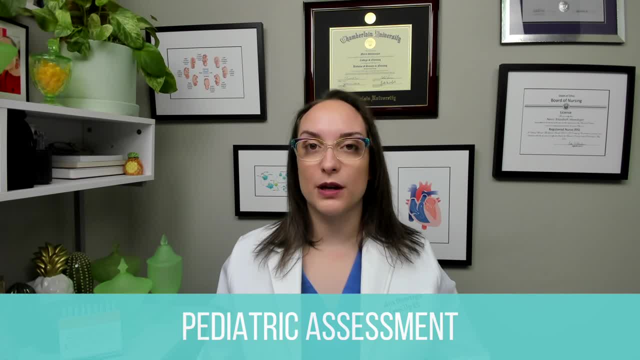 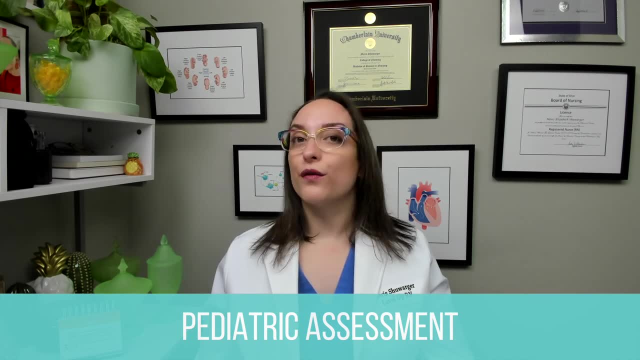 although that may change. So I'm going to be talking to the caregivers and not to the child themselves, but I'm going to be asking things about their family history, medications that they take, personal health history, But other things that I may be asking about. a child versus an adult would. 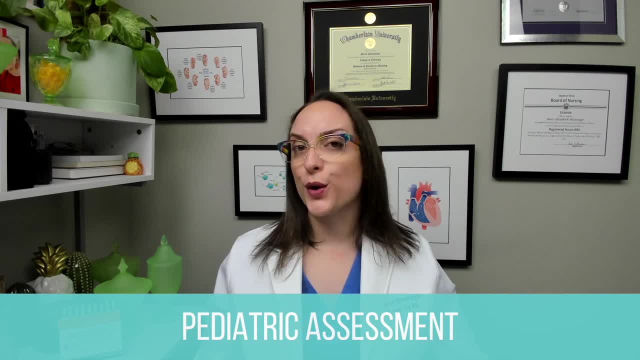 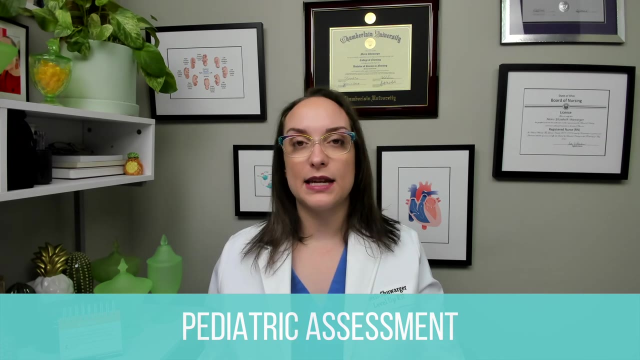 be about their birth history as well. Were they born prematurely? If so, how premature? Did they spend time in the NICU? Did they have any sort of birth trauma? All of those things are important for us to know about a child because it can change what we expect to see and what we might. 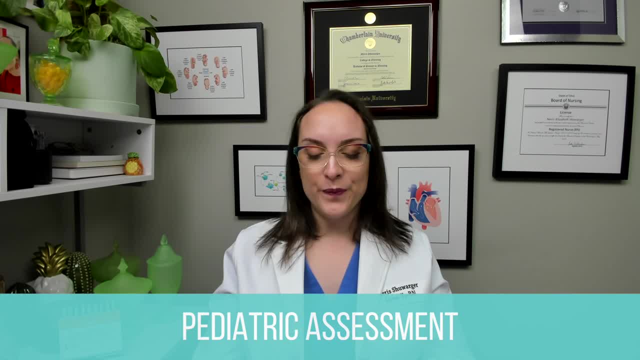 need to delve into further for the child now. Now, other things that we may need to know are going to be their immunization status. right, We're going to ask adults this too, but it's important for us to know where a child is in their immunization status. Are there any that they 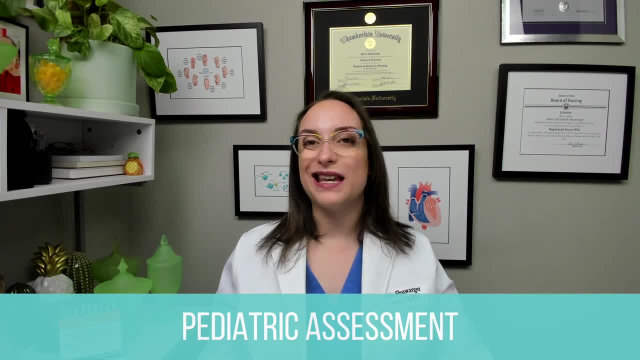 haven't received. Are there any that they are behind on? Do we need to catch up That sort of a thing? Now, one thing that I do want to point out here on this list is the order of vital signs. This is especially important when we're thinking about very small children, because they get 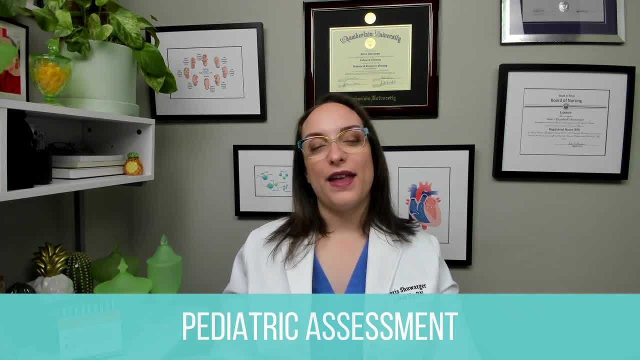 agitated easily and start to cry, And when they cry their other vital signs can be affected. So, first off, we want to count the respirations before we ever touch the child. right When they are nice and calm and they're hanging out with mom or dad or a caregiver, we're going to count. 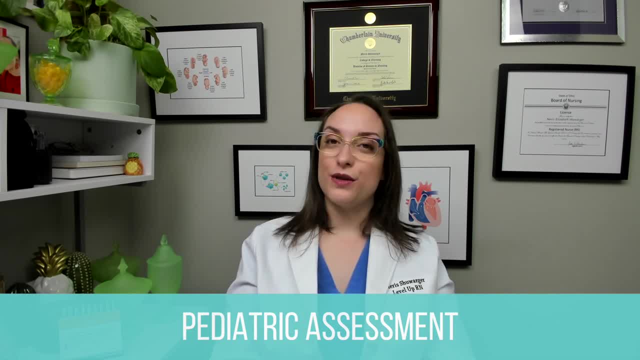 their respirations first. Then we're going to do the apical heart rate And then, if indicated, we're going to do a blood pressure. This is not always indicated for children. This is not something that we're going to do routinely, only if we have a reason to be doing it. 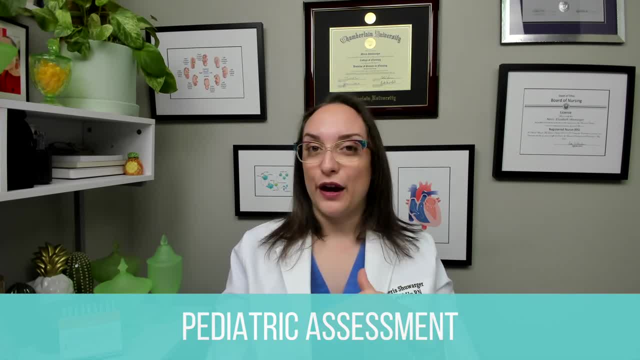 And then, lastly, we're going to do temperature. If you've ever taken care of small, small children, infants, they lose their minds when you take their temperature. You put that probe underneath their arm and they start screaming. So that is something that we are going to do last for sure. 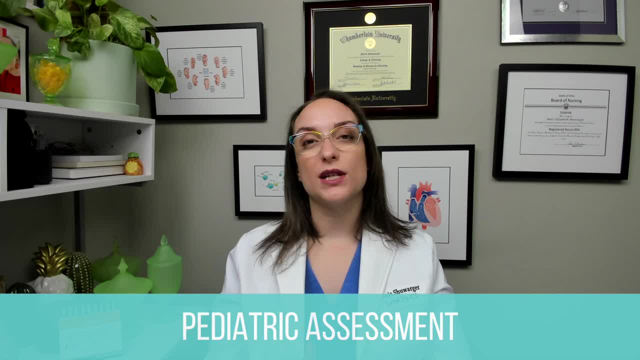 Now pain assessment we're going to talk about in a minute, but we need to make sure we're using appropriate scale. And then, when it comes to their physical growth and development, we're going to measure a bunch of different things. First, of course, we're going to measure. 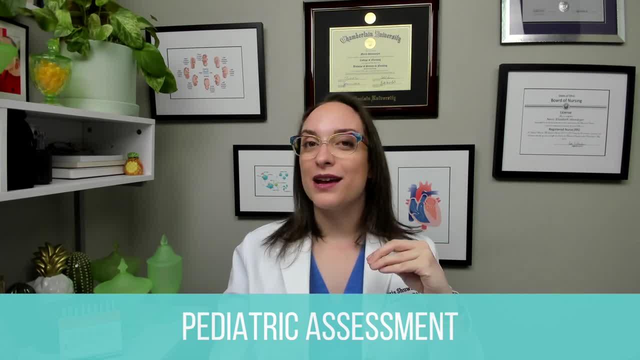 their length or their height. It's the same thing, but we call it length when a child cannot stand upright. It is height when they now are able to stand upright. So same measurement, different word. We're going to measure their weight and their head circumference. Again, this is typically 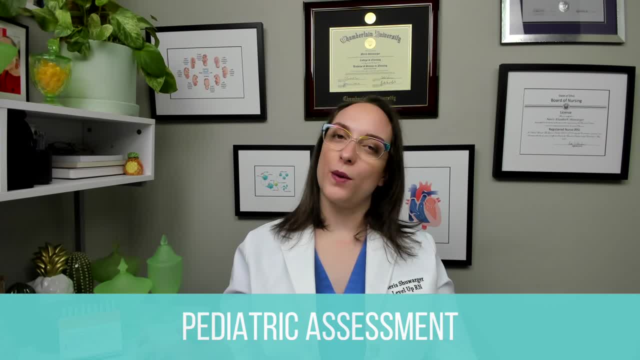 for younger children. We're not going to do that for older ones, but we are going to do that for the younger ones who are going to assess their fine and gross motor skills, And we typically are going to ask questions about other developmental skills as well, like the number of. 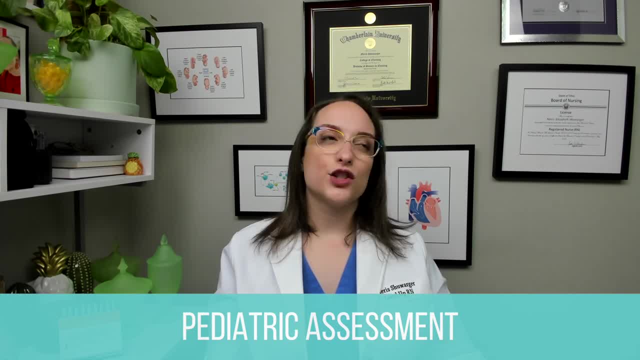 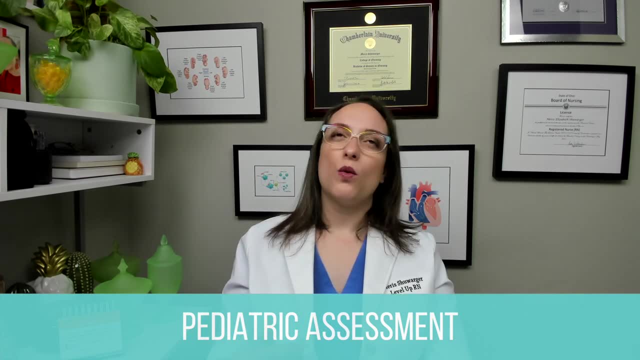 words that they might know? Do they do certain things? Do they smile at you? Do they make eye contact? All of those things will be assessed as well, And, along with their cognitive status and their psychosocial development, we're going to assess all of that. 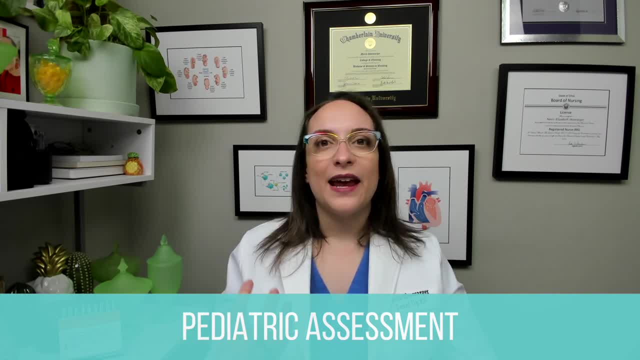 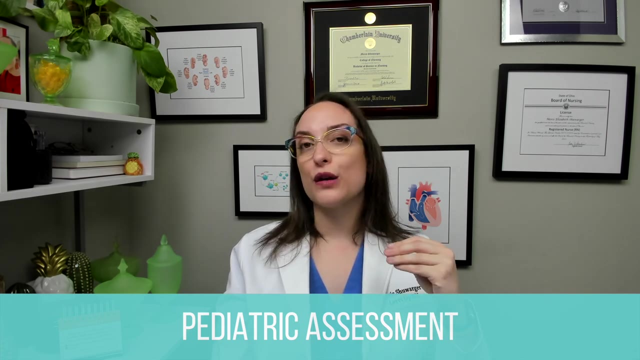 Let's do anthropometric data, which means the data of the physical body: the height, the weight, the head circumference. All of those things are going to be plotted onto a graph, but it's important to remember to use the correct graph. There's one for boys, for girls, for different. 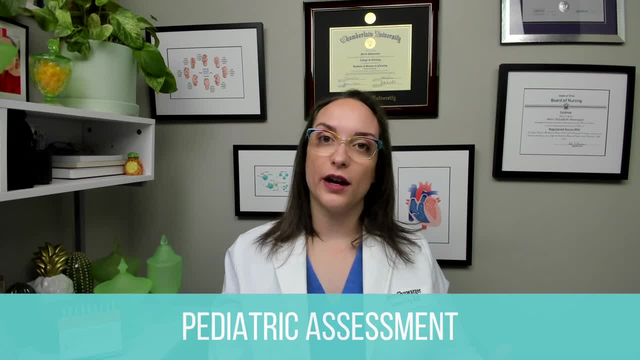 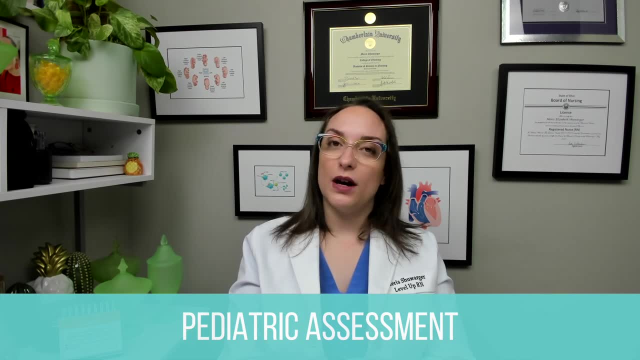 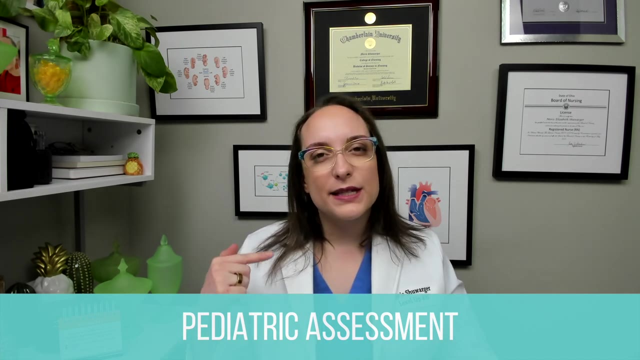 diseases. If we know that a child has a certain condition, we need to plot them on the correct graph for that condition, And there's also charts based on ethnicity as well. Now, the thing that matters most is not the specific number, but rather the trend. So if my child is in the 15th percentile for height and the 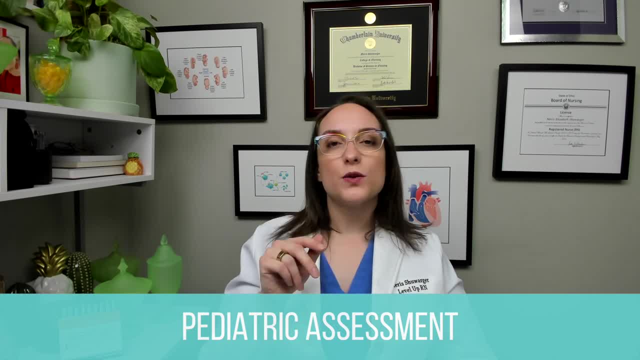 20th percentile for weight. that's cool. We just want to see: are they staying in those same kind of ranges, plus or minus a little bit, Or are they suddenly dropping drastically or going up drastically in that range? And we're going to ask those questions And we're going to assess. 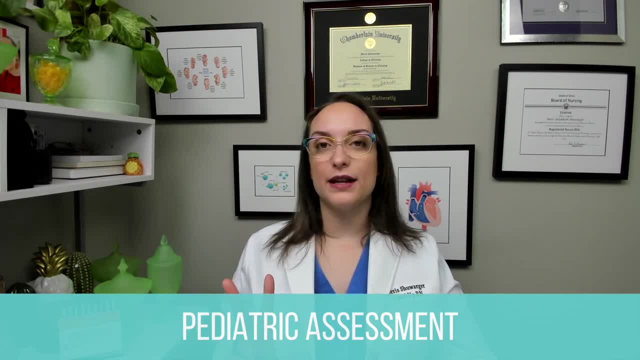 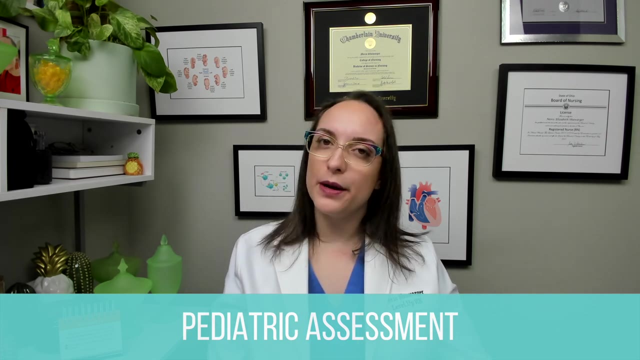 that percentile. But there are two things that we do need to assess further. A child who is less than the 5th percentile or greater than the 95th percentile needs further investigation. It doesn't necessarily mean something is wrong with them, just that we need to investigate further to make. 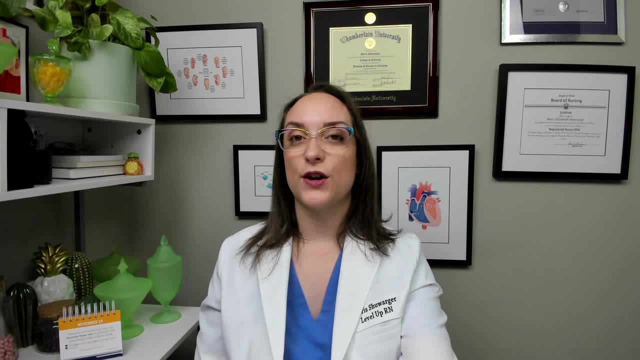 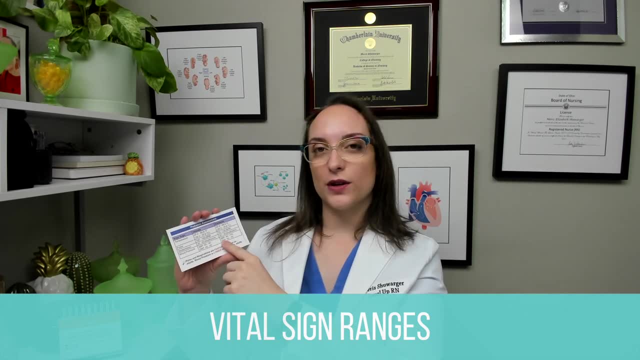 sure everything is okay, All right. moving on, we're going to talk about expected vital signs. So on, here we have this very nice chart for you. We have the vital sign infants and children here, because infants have slightly different vital signs than children. 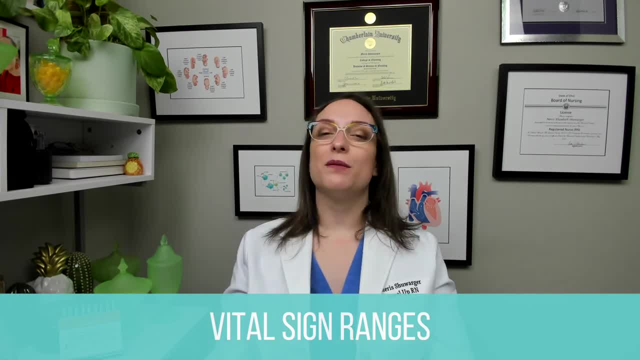 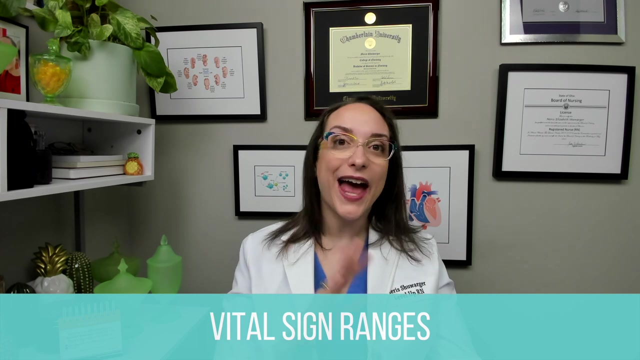 who have slightly different vital signs than adults, So it's important to know each Temperature. luckily it's the same for both 97.4 to 99.6 degrees Fahrenheit, or 36.3 to 37.6 degrees Celsius. Now, in infants, the normal pulse range is 100 to 160 beats a minute. That is very. 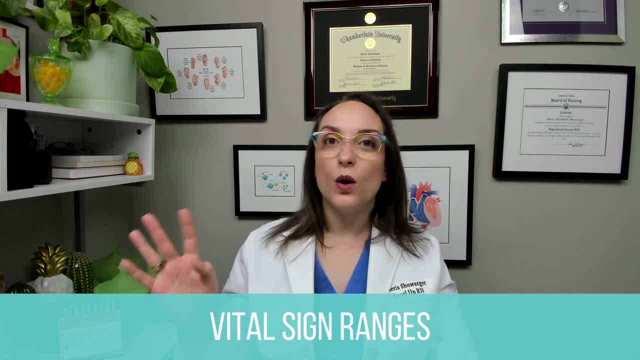 fast. If an adult had a heart rate of 160 beats per minute, we'd be thinking that they need like cardioversion right. Very, very important to know. they are expected to be much higher. Children, though. their range is a little bit lower than that. They're going to be 70 to 120. 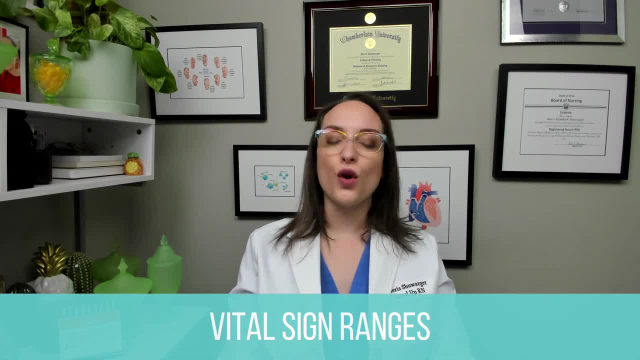 beats per minute, still higher than adults. right Respirations of infants are expected to be 30 to 60 breaths per minute, whereas in children it's 20 to 30 breaths per minute. And lastly, blood pressure In infants, the systolic blood pressure, and you're going to. 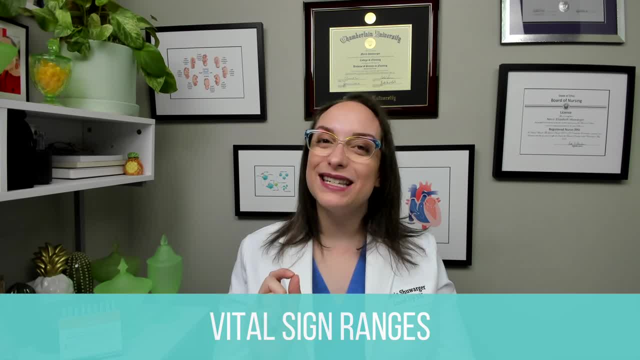 think I'm wrong. the systolic blood pressure is 65 to 90, and the diastolic blood pressure is 45 to 65. If I had an adult patient with a pressure of 65 over 45, I would be absolutely panicking. 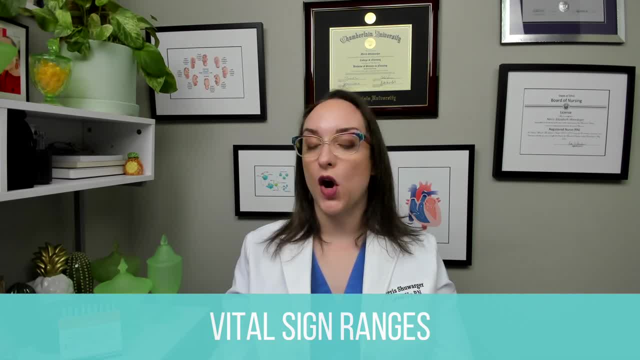 right, But this is normal for an infant. Now, when we're talking about the blood pressure of a child: systolic 90 to 110 is the normal range. diastolic: 55 to 75. So we do have a nice key point here to. 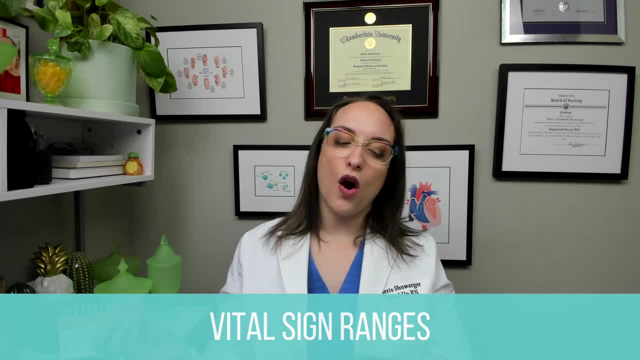 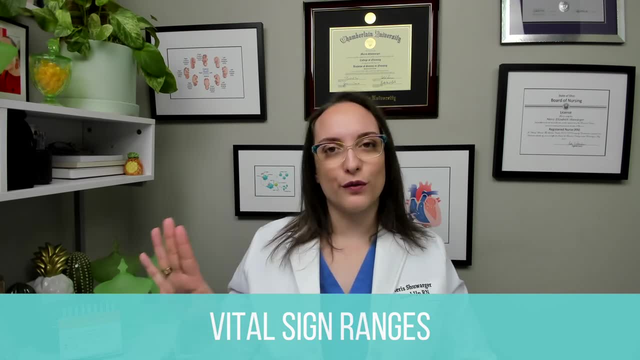 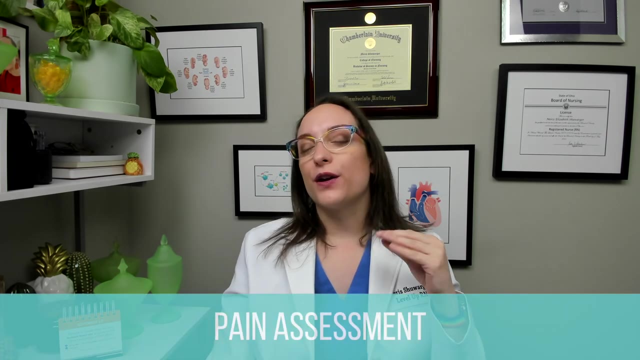 help you remember. Pulse and respirations are faster in children versus adults, but blood pressure is lower. So everything is going to be elevated, except for blood pressure is going to be lower, right? Lastly, we're talking about pain assessment. It's very easy for me to ask you as: 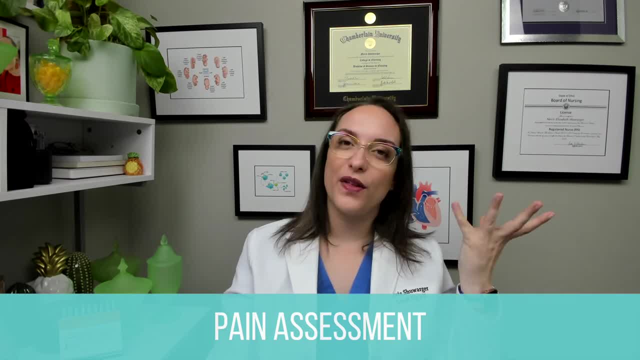 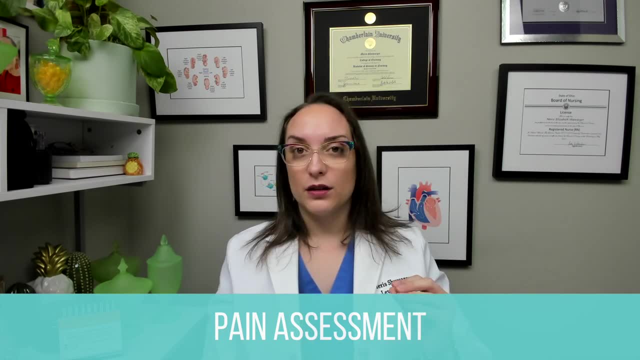 an adult to rate your pain. If you're an adult, you're going to have to rate your pain If you're from zero to 10, right, we have that sort of abstract thinking. We can think in terms of putting my pain into a numeric form. A child can't and an infant certainly can't, right? So 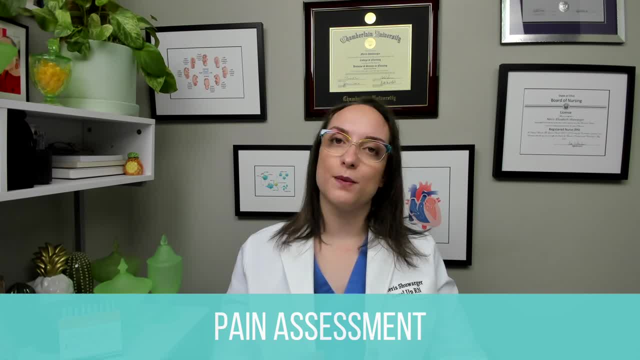 we have had to adapt to different ways to assess a child's pain. We have a bunch of different scales for you. I'm going to hit some of the major ones here. The cries scale: well easy to remember who this is for. It's for neonates, preterm and full term. Who cries? 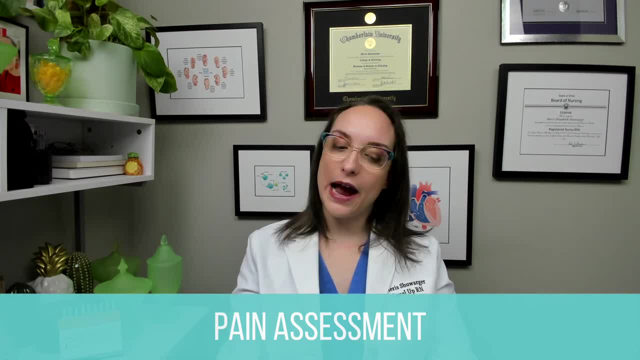 Newborns, right Neonates. they cry, So that's the cry scale, The FLAC scale F-L-A-C-C. that stands for face, legs, activity, cry and consolability. So who is that? for? It's for two months to seven. 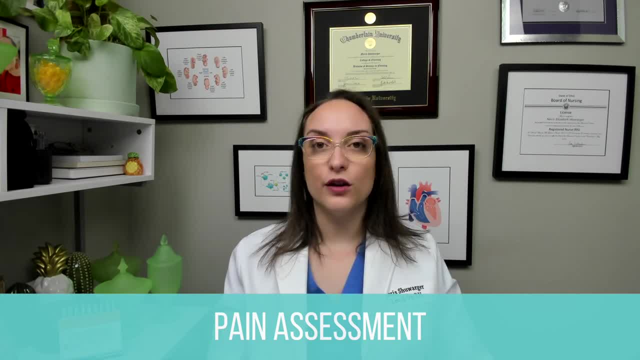 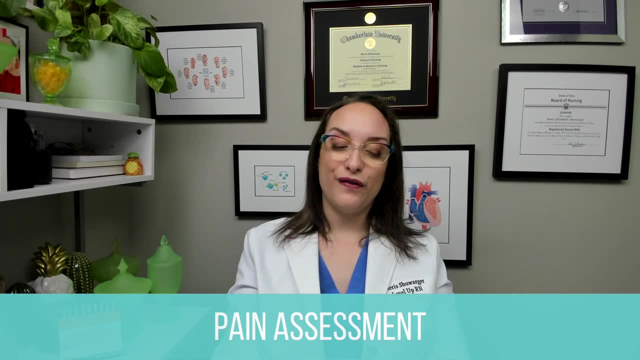 years of age. Now the faces scale. This is the one that I personally have seen the most in my clinical practice when we're talking about children. This is the faces scale. This is six drawings of faces To rate pain from a scale of zero to five. but this is used for anyone who is greater than or. 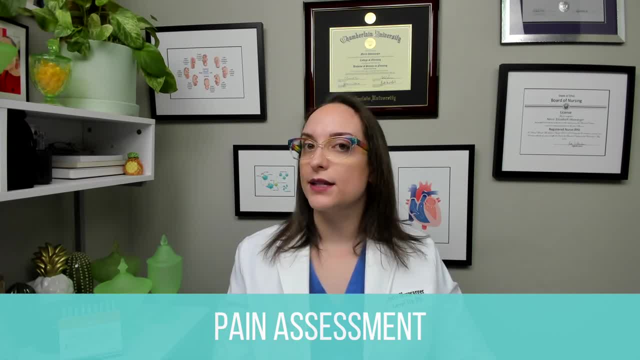 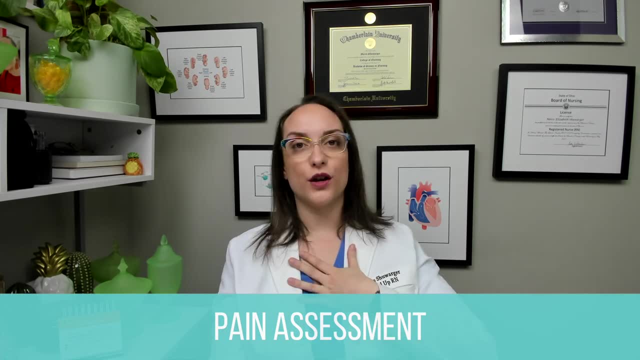 equal to three years old, They can use the faces scale. Outcher is for three to 13.. And then the numeric pain scale. what we are used to Tell me about your pain, Zero being no pain, 10 being the worst pain you've ever experienced- That's numeric pain. 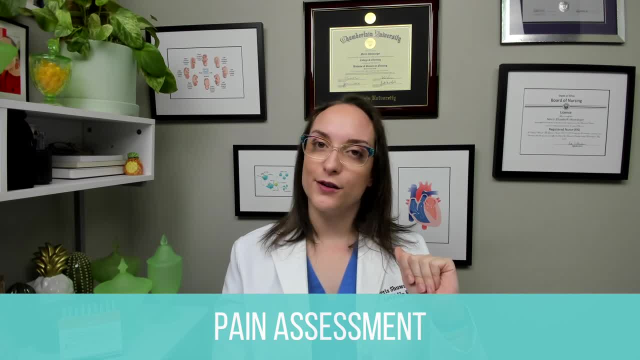 scale, and that is for children greater than or equal to eight years old. Personally, I would be using that more for older children. I would be using that more for older children. I would be using that more for older children as well, who have that ability of abstract thinking. I myself- 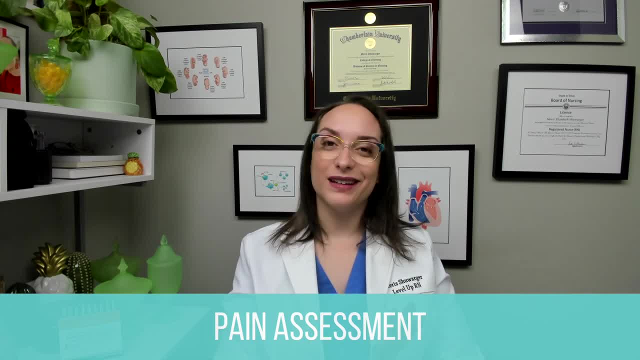 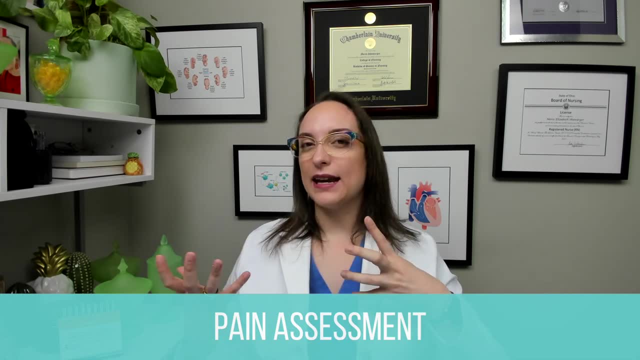 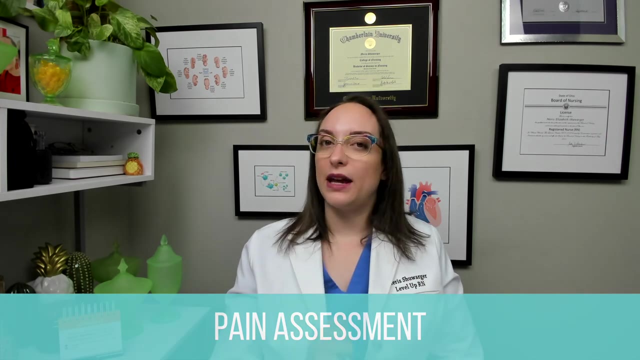 would say probably 11 years, but per the terms of the scale, anyone over eight can use that scale. But just remember, turning pain into a number is a really logical, abstract sort of way of thinking. Little kids are not going to be able to do that. All right, I hope that review was helpful for you. 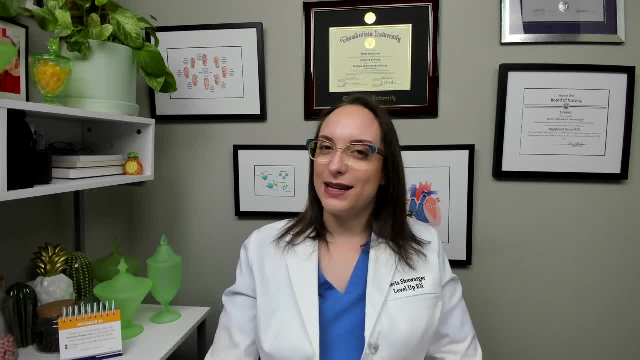 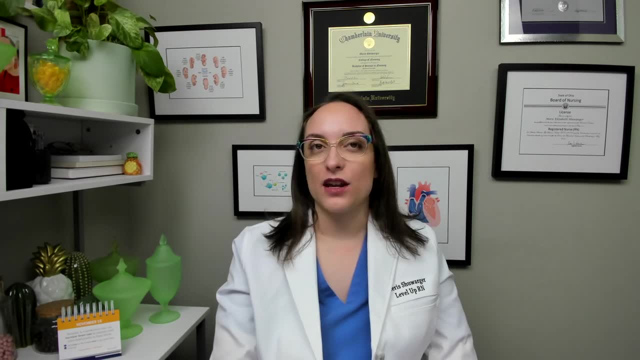 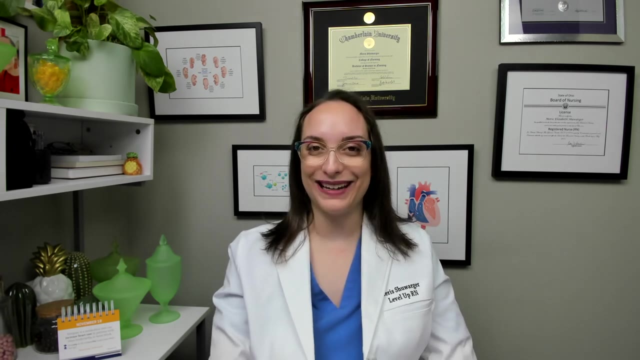 Stay tuned because I have some quiz questions for you To test your knowledge of some key facts I provided in this video. Okay, So first up, which vital sign should the nurse obtain first when assessing an infant? What is the first vital sign to obtain? 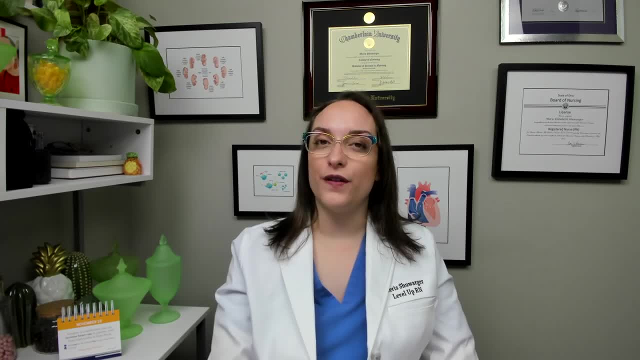 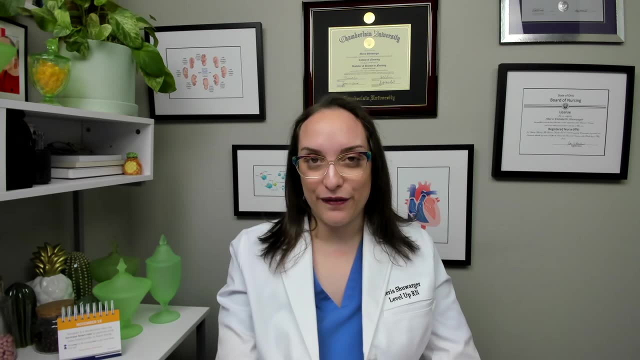 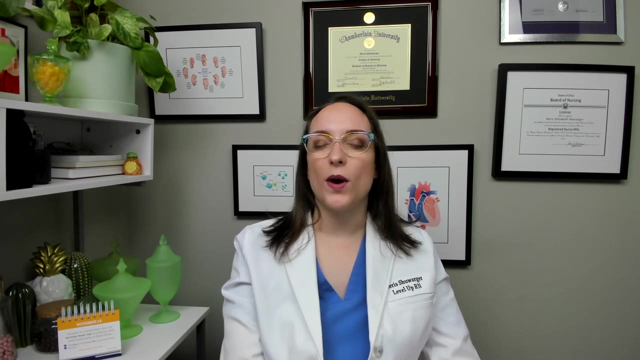 Next up. I want you to tell me which of the following- select all that apply. which of the following vital signs are out of normal limits for an infant? Okay, BP 72 over 50, respirations: 25 breaths per minute.